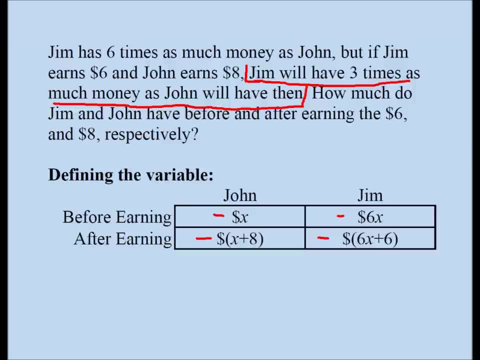 But I'm not interested in that. I am interested in the new amount. And here Jim is three times as much as John, Only three times. So Jim's amount is 8x amount is 3 times John's amount. So whatever Jim has now is equal to 3 times that And 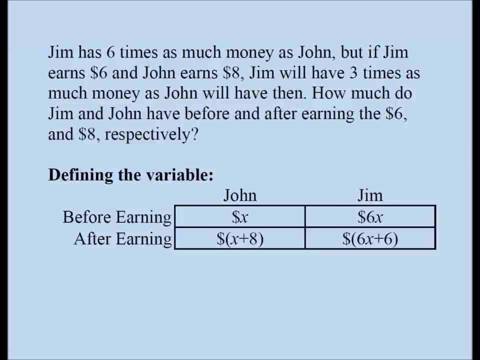 let's erase everything and write this down. So setting up the equation- this is my equation: Jim's amount is. this means is or is equal to 3 times John's amount. That's exactly what this says, this line Again. you want to pause the video here and really reflect The question. 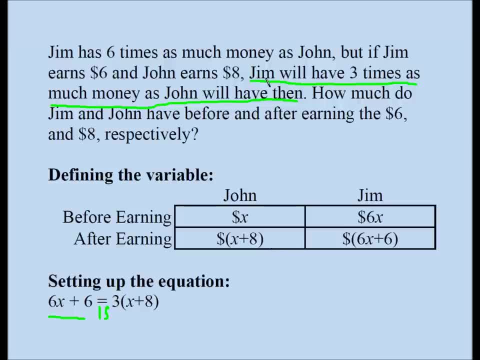 says, after they earn the money, 2 amounts, Jim will have 3 times of what John will have. That means this is equal to 3 times this. 3 times this, That's what it means. So once we have the equation, the equation is not very complicated. 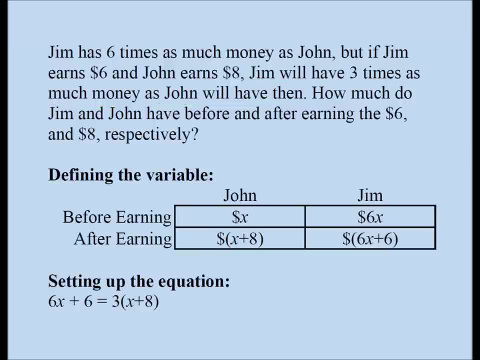 We will just go ahead and solve it. Let's solve this equation. This equation: 6x plus 6 is equal to 3x plus 8.. Let's move on. Go to the next slide. Okay, this is my equation. 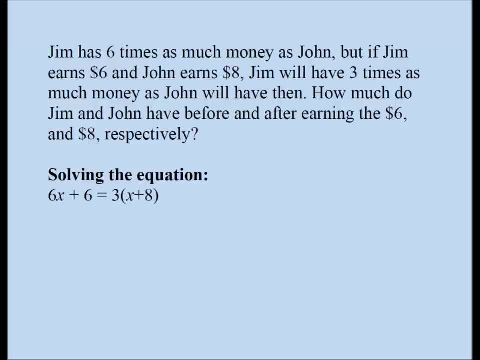 from my previous slide. So what can I do next? I distributed 3 over x plus 8 and I get 3x plus 24.. I moved my variables around. I subtracted 3x from both sides. I moved my variables around. 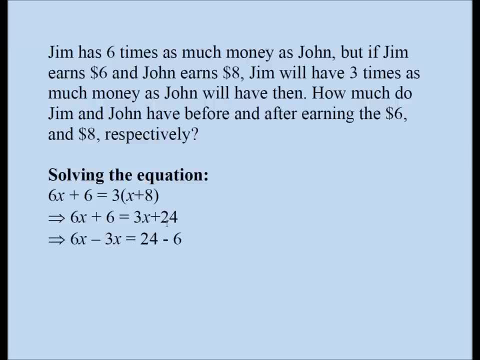 I have 6x minus 3x on the left hand side and subtracted 6 from both sides, and I have 24 minus 6 on the right hand side And 6x minus 3x is 3x. 24 minus 6 is 18.. I divide both sides. 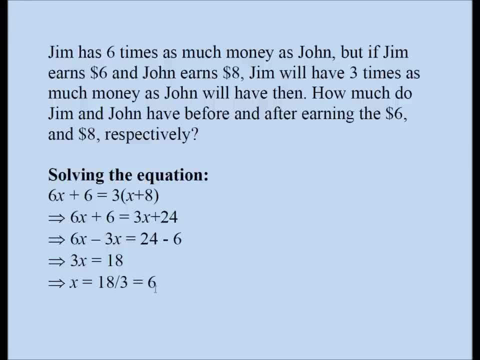 by 3 and I get x turns out to be 6.. That's the value of x. Now we're going to go back and answer the specific question that this question wants me to answer. They want us to find out how much money did the two guys have before and after they made the money?